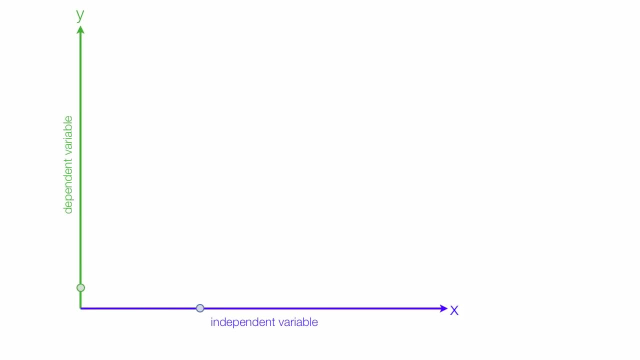 If they move in the same direction. if the independent variable increases and the dependent variable increases as well, like this, we say there's a positive relationship. If, on the other hand, as the independent variable increases and the dependent variable decreases- like this, we say there's a negative relationship. the line would look: 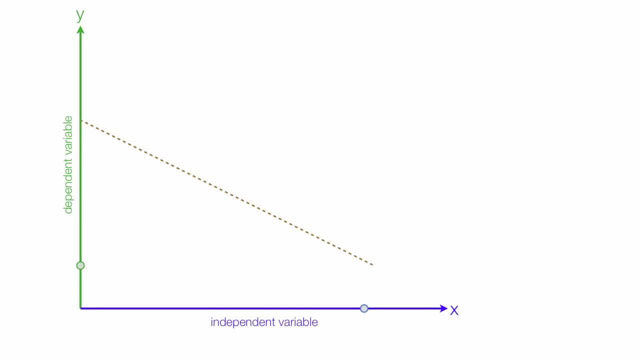 like this Go downward In linear regression. we try to make a line a line. to make a linear regression, the key is on line, right there, a straight line. want a manufactured line, Right, Okay. So before we do something, 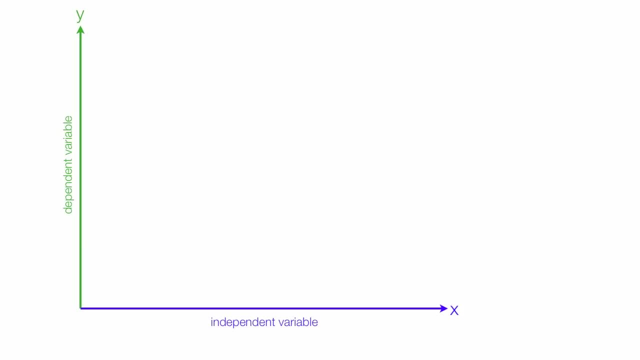 straight line. You can also do curved lines, But for the this topic it's all straight lines. To actually conduct regression, I take observations And I'll just plot some more observations in here randomly. I'll stick them in here like that And I try to find. 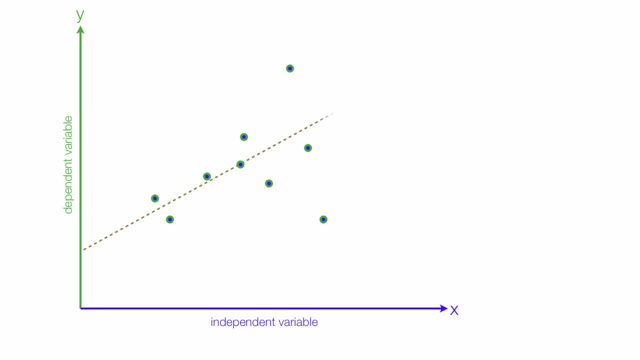 a line that will fit, a straight line that fits to all these different points, And this is called my regression line And it's based upon the least squares method And in the end, I want to minimize the difference between the estimated value and the actual value. 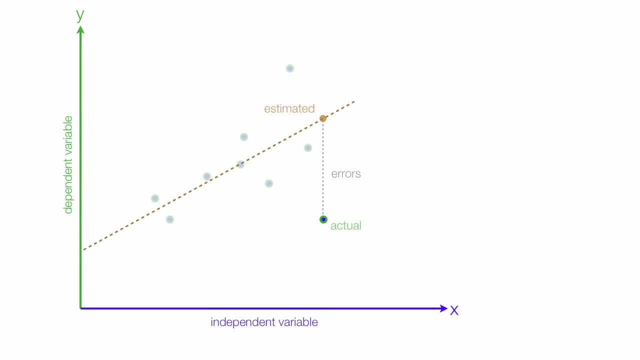 I want to minimize my error errors. This line will have a lot of errors if I compare the actual to the estimated value. And again the point is to minimize these errors or make them as small as possible. Now let's imagine I put study time on the x axis, or make that. 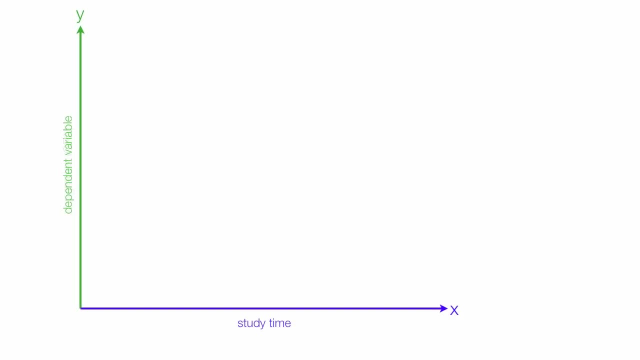 my independent variable And the dependent variable becomes grades or GPA. As study time increases, grades should go up. there is a positive relationship. In regression. we develop these equations like this. In this case, y hat is estimated grades and it's based upon: 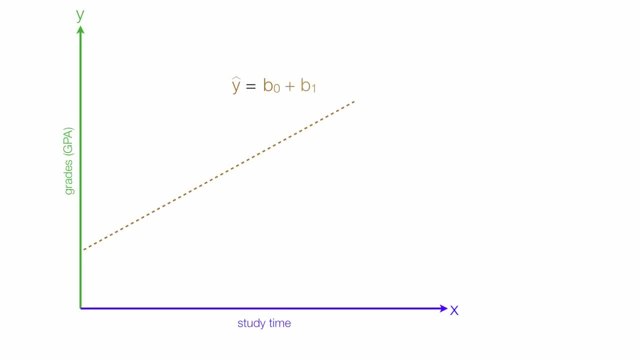 or it's equal to b naught plus b one times x, Where x is study time, B not. we derive mathematically and it is the y intercept B one. we also derive mathematically and I'll do in a later video, And it's the slope of the line In this case. 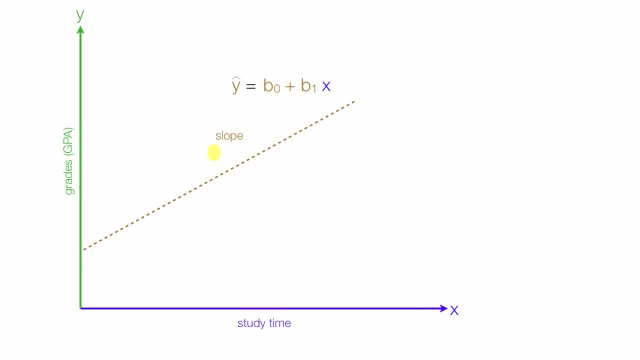 the slope is positive. In the next video I'll discuss how you develop these equations. Now, if I change the x axis to time on Facebook, we see a negative relationship. More time on Facebook, grades will suffer and go down. a negative relationship. What we're estimating? 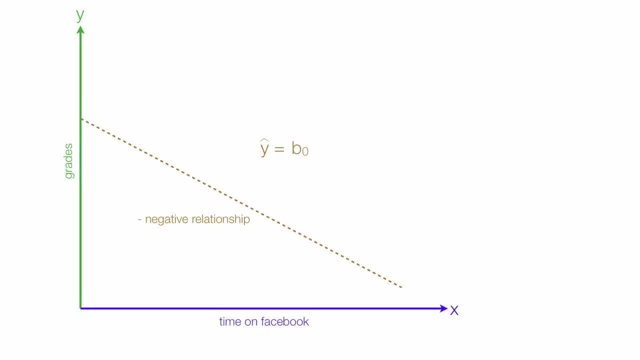 is still grades. estimated grades is equal to b naught minus b one times. x or x is time on Facebook. B not is still the y-intercept. the y-intercept and it is a calculated value. the slope of the line is negative. b1 because it's downward sloping. negative relationship. 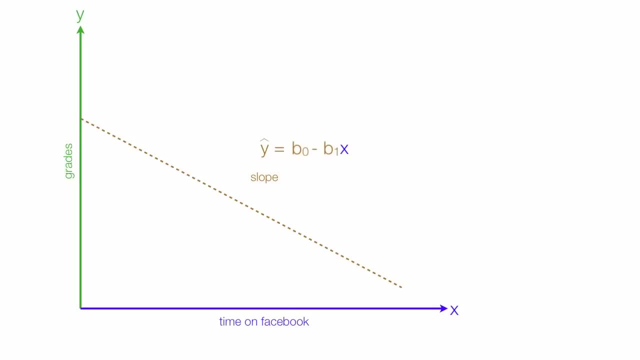 and, as I said before, I'll show you how to calculate this equation in the next video. the X is the independent variable, the Y is the dependent variable. the X is what we control, what we manipulate, what we change, and the dependent variable is the outcome. so study time is the independent variable, it's what we control and 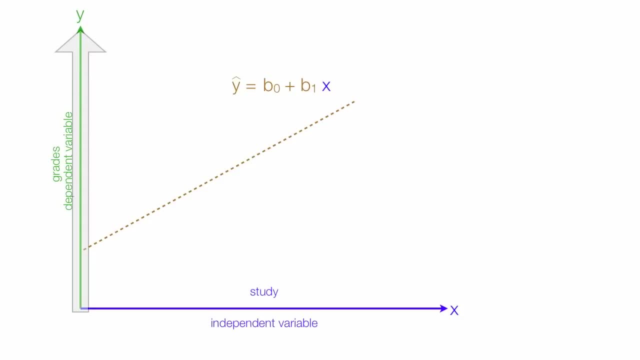 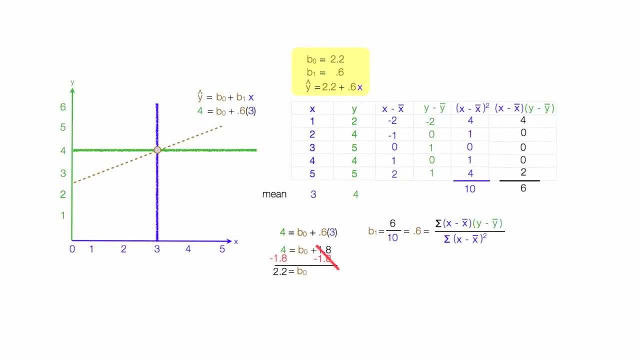 manipulate and your grades are dependent upon how much you study. now this looks really ugly and it's what I'll talk about in the next video, but I'll step you step-by-step through it and hopefully make it simple for you.